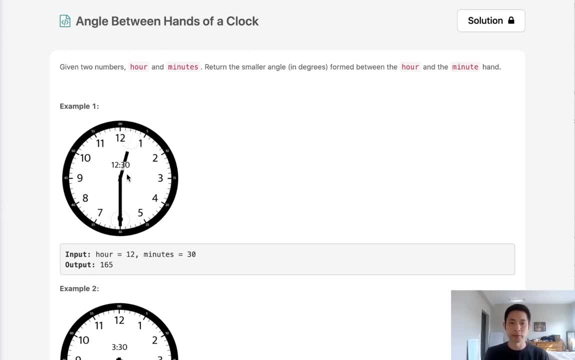 want to return 165 because that's the number of degrees between them. That's the smaller one anyway. On the other side it would be actually 195, but we want to return the smaller one. If we're given 3 and 30, we want to return 75 because that's the smaller amount. 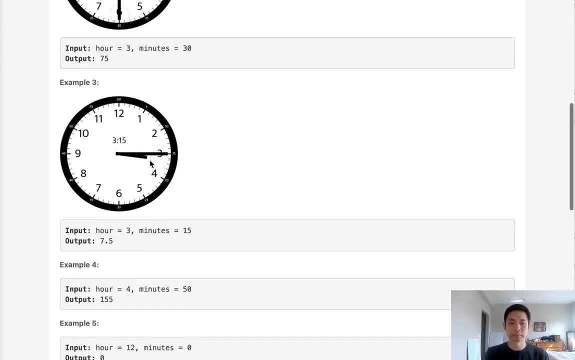 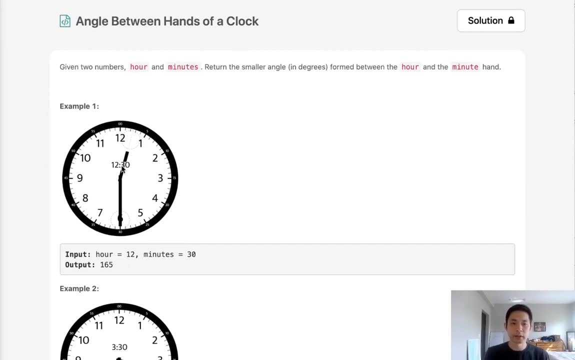 of degrees and so on and so forth. I love this problem because it's practical. It touches upon different areas. It's not just a computer science problem, right? It's also a math problem, so you might need to remember your geometry. So the first thing is how many degrees are? 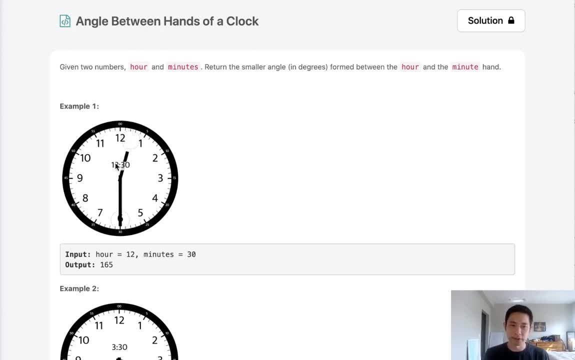 there in a clock. Now it's a circle. obviously There's 360 degrees right. But there's a couple gotchas here. First, the hour hand will change a little bit depending on where the minute hand is. Now the minute hand itself. 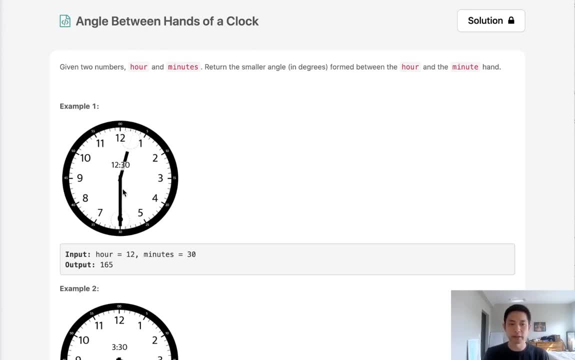 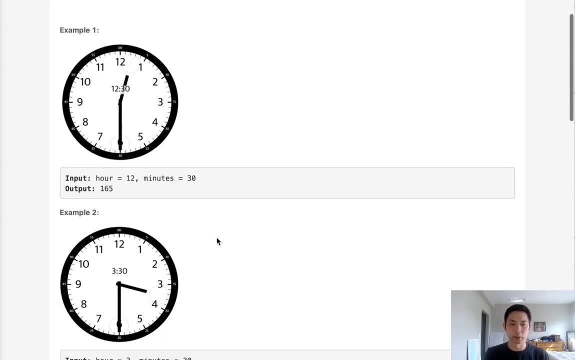 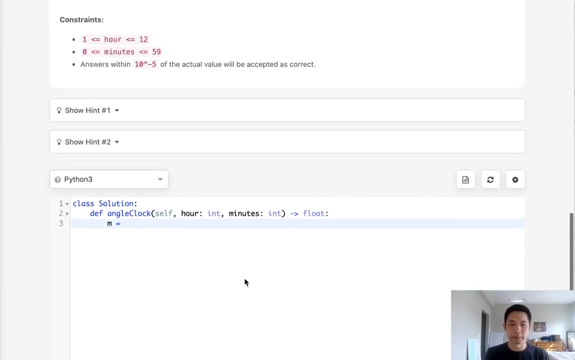 doesn't care about the hour hand, So we should start with that. Let's say how many degrees will the minute hand be at given whatever number we're given? So let's start with that And I'm going to just call it m. This is the number of degrees for the minute hand. 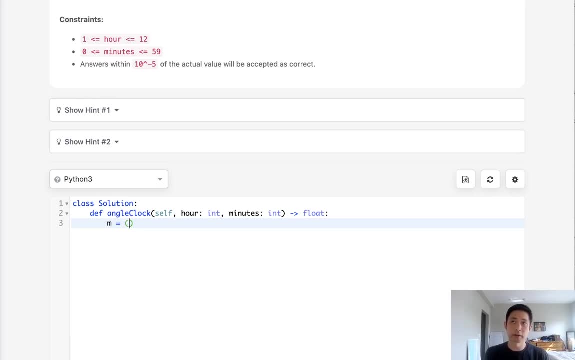 So to get that, how many minutes are there in an hour? There's 60 minutes, right? How many degrees are there inside of a circle? There's 360.. So basically, every minute is going to be 6 degrees and we can figure that out by 360 divided by 60.. Now we just want. 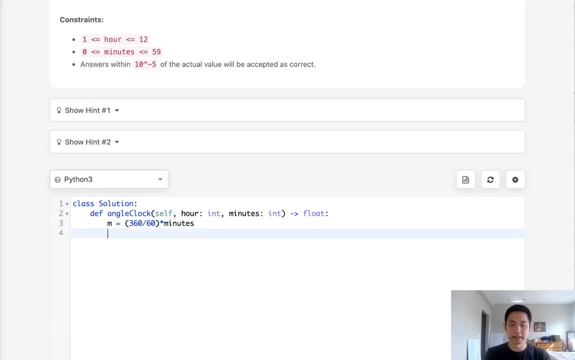 to multiply it by the number of minutes And that's going to give us the degree for the minute hand. Great, Now what about the hour hand? Well, the number of degrees on the hour hand. there's going to be 12 hours. 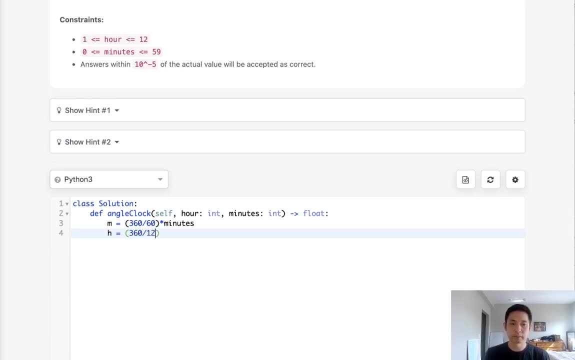 in a clock, So 360 divided by 12.. I'm actually not sure what that is. I think it's 30 times the hour. But hold on. It depends a little bit, or it also depends on what the minute hand is going to be at. 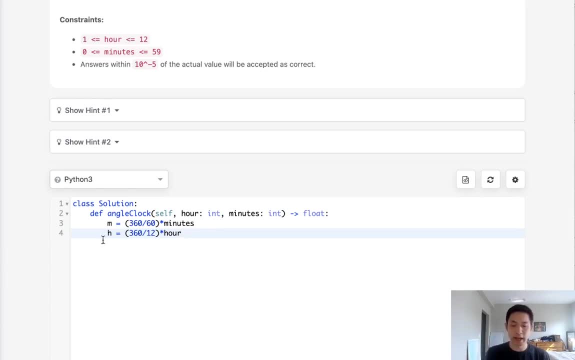 So, depending on where the minute hand is, we need to add a couple more degrees for the hour hand. So how do we do that? Well, let's think. First, let's find the fraction of how many minutes it's at. So since there is 60 minutes, we can say minutes divided by 60.. 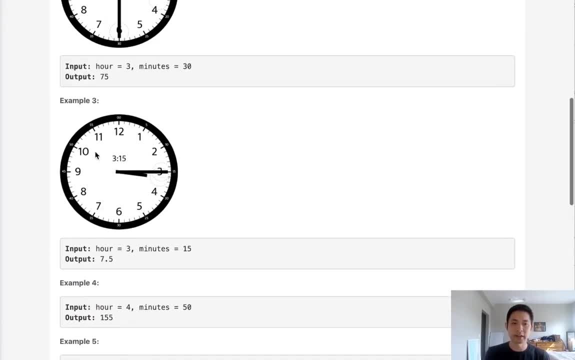 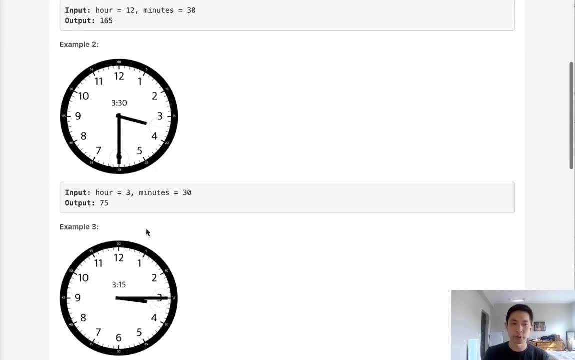 That is the number of minutes divided by 60.. That is the number of minutes divided by 60. That is the amount that it's at around the clock. So if it's at 30, that would be half. If it's at 45, that would be 3 fourths and so on and so forth And really all we need. 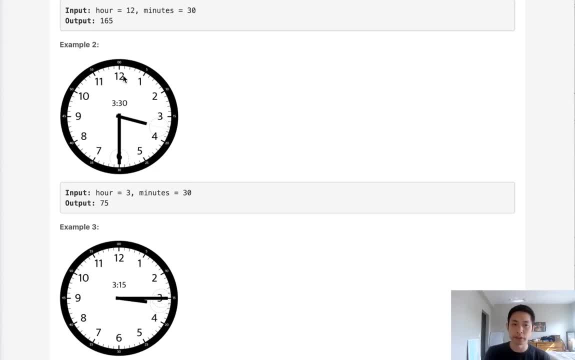 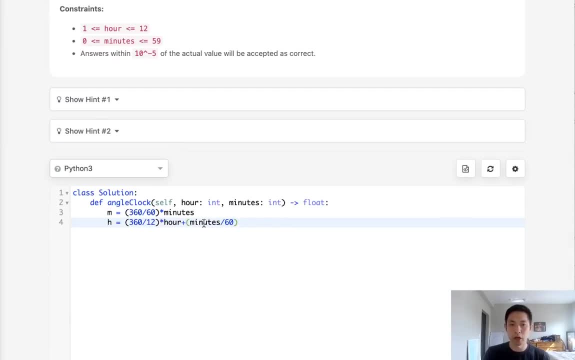 to do is add that fraction amount to however many degrees there are between hour to hour, And, if you recall, that was 30 degrees, right. So all we need to do then is multiply this, the minutes divided by 60, times however many degrees there are within an hour to hour. 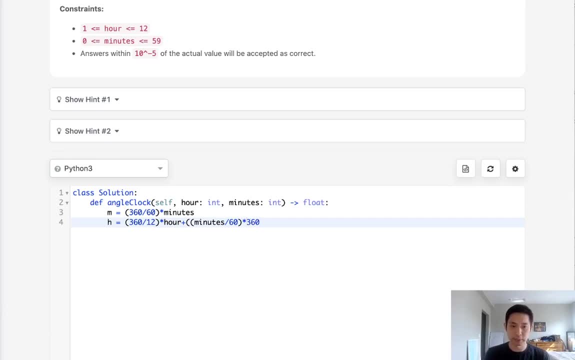 Which is 30. And we could, just to be explicit, say 360 divided by 12.. And that should give us the degree for hours. Now, the difference, What is the difference between the two? Well, this is where it gets a little tricky, because it depends whether the hour hand is ahead. 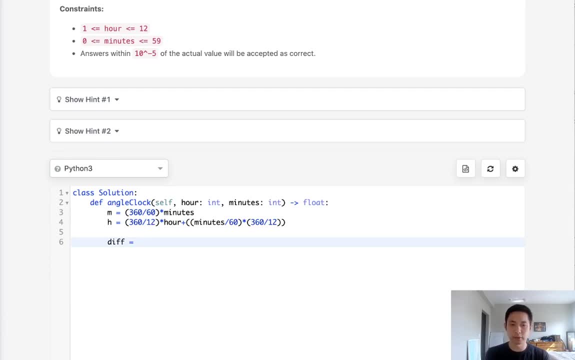 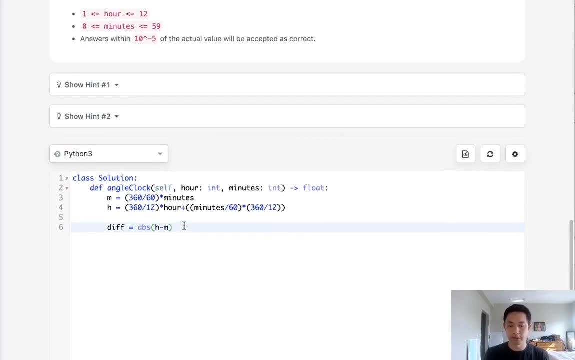 or the minute hand is ahead, right, But we can find the difference by simply getting the absolute value. It doesn't really matter which one you pick, So that would be the difference. So you might think, okay, we can just return the difference here, But no, we can't because of what I mentioned. 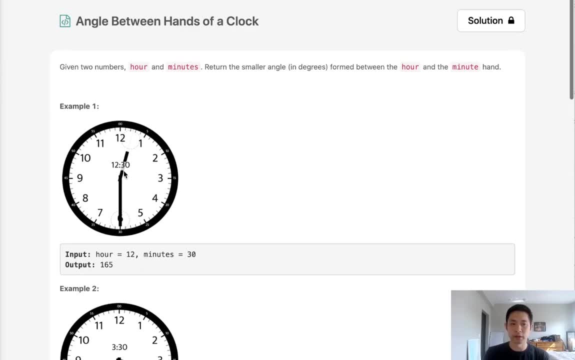 earlier, We might possibly be getting the other side. We want to get the shorter distance. So, depending on which side we've calculated, we're not sure right now, But to get the other amount. so say that we've calculated this degree, this would be 195.. Let's get the other. 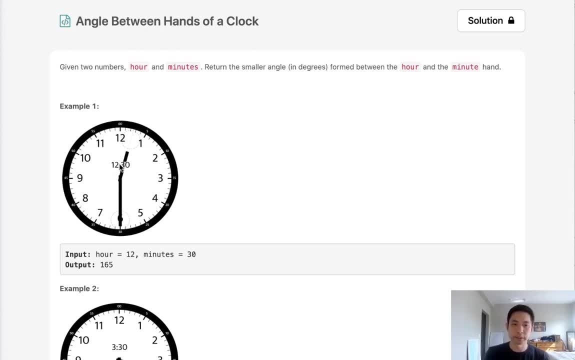 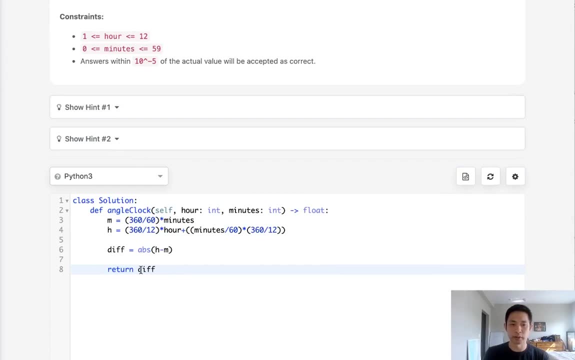 side, And all that would be is 360 degrees subtracted by whatever we calculated here. Okay, so that would mean we just return the minimum between the diff and 360 degrees minus the diff. So whatever is the minimum here, that's what we should return. Now let's submit that. Let's.